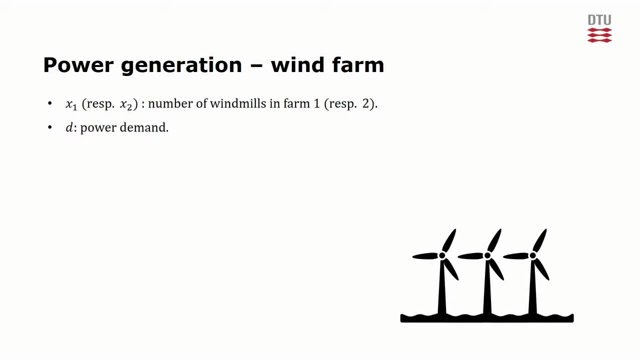 distribution. It might not be the same for windmills in each of the two parks. Parameters w1 respectively. w2 represents the amount of power generated from an algorithm'd wind situation from the wind environment to an environmentalCause average windmill in wind farm: 1, respectively 2.. 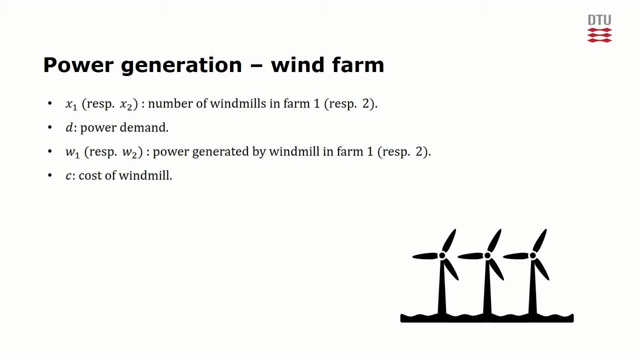 There is a cost associated with buying and setting up a windmill. This cost is given by C, independently of which wind farm the windmill belongs to. A windmill has an expected lifetime which has been taken into account in C, such that C is the per year cost of the windmill. 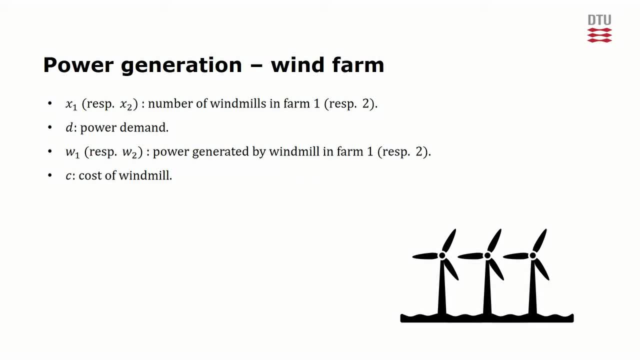 The objective is to minimize the total costs while satisfying the power demand of the city. When the wind farms are set up, the number of windmills cannot easily be changed. Instead, as a recourse action if the demand is not fully met by the new windmills, a set 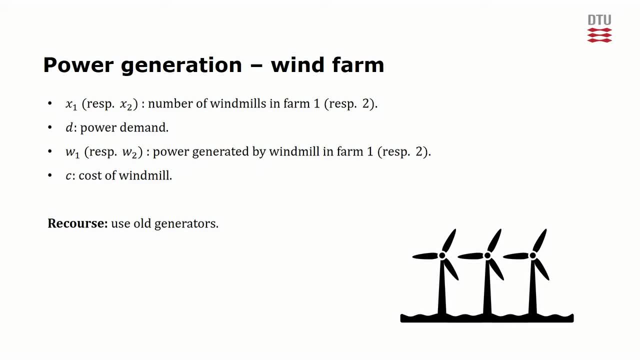 of old generators can be used to generate the remaining demand. However, using the generators will be expensive and the city will be penalized for not fully living up to the new green energy requirement. The problem is often solved in the beginning, as we have already said. 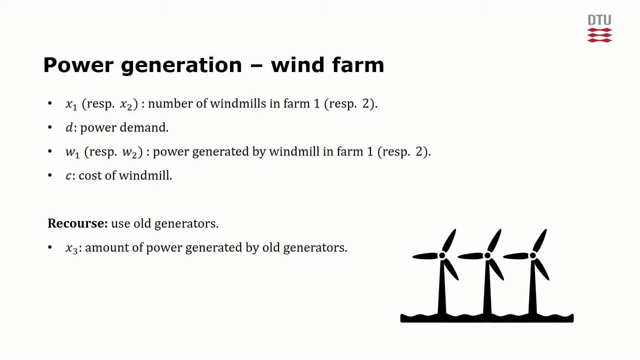 We introduce the continuous variable X, which corresponds to the amount of electricity generated by the old generators. We also introduce parameter O as the per unit of electricity cost associated with using the generators. This also takes the monetary penalties into account. In summary, the problem has two stages. 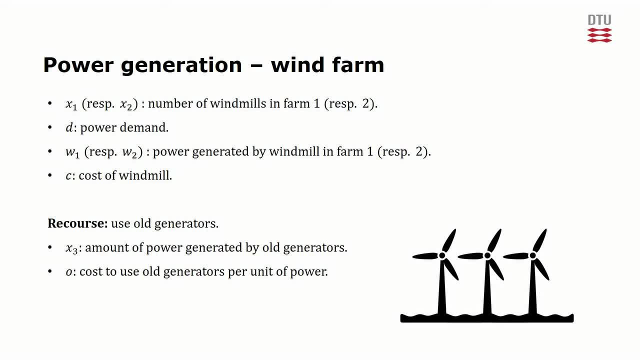 The first being to determine the number of windmills in each of the two wind farms and the second being to determine how-to. This is one of the most common ways of solving this problem. much electricity to generate with the old generators. we are now able to write up the. 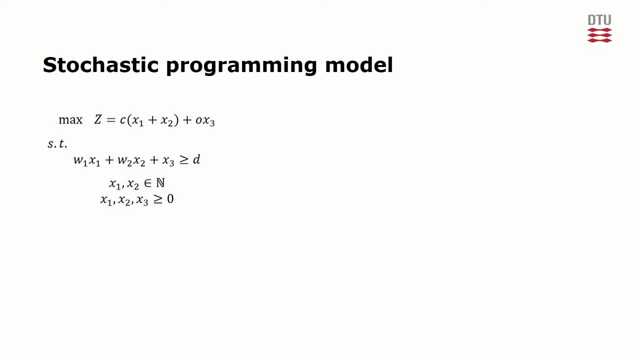 stochastic programming model. the model is actually quite simple. it has a single constraint that ensures that demand is satisfied and the objective simply sums the total costs, including that of the old generators. because we do not have a limited number of scenarios, we can instead use simulation to generate a number of scenarios using the probability distribution of w1 and w2.